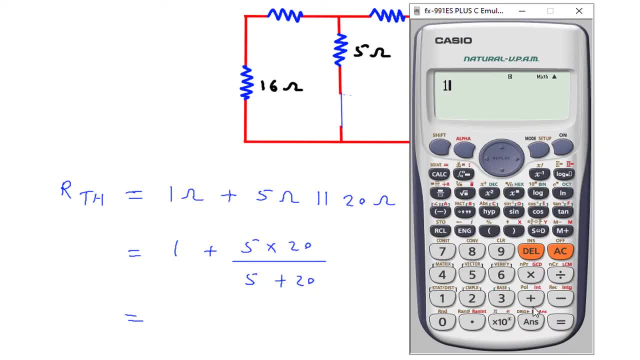 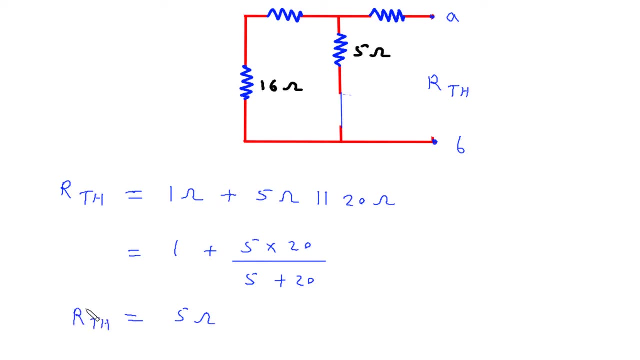 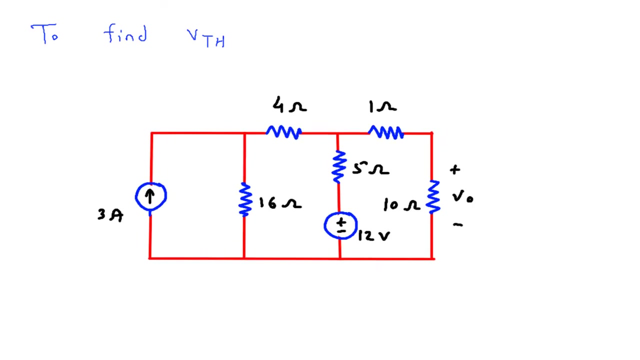 This will be 1 Ohm 1 plus 5 into 20, divided by 5 plus 20, so it is 5 Ohm Rth is equal to 5. Ohm Rth is Thevenin's resistance. next we have to find Vth. so to find Vth, we will consider this. 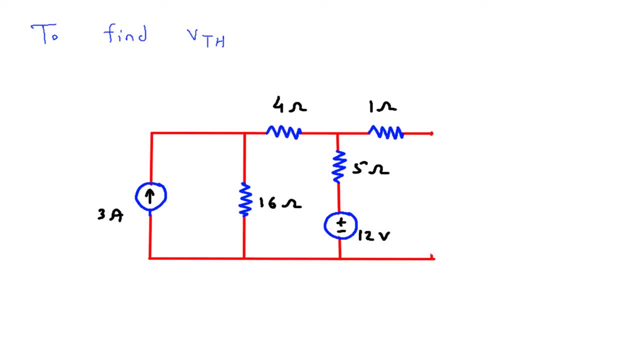 circuit. this is terminal, this is terminal A and this is terminal B and this is Vth. so this will be positive and this will be negative. now here, this will be Vth. let's say this is node V1,. let's say this is ground node with zero voltage. this is current I1,. 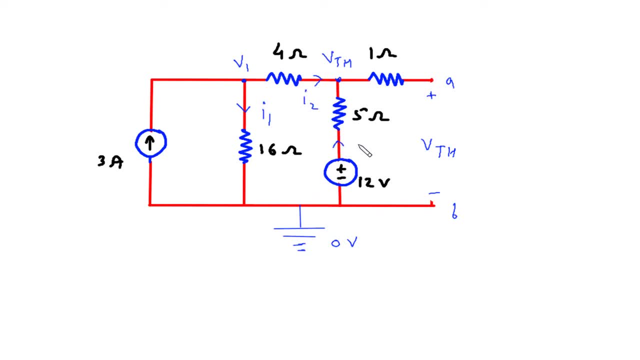 this is current I2 and this is current I3.. Now we will apply KCL at node V1.. Apply KCL at node V1, so entering current at this node is 3 Ampere. leaving current is I1 plus I2, I1 plus I2, I1 is V1 minus 0 by 16, I1 is V1 minus 0 by 16 plus I2, I2. 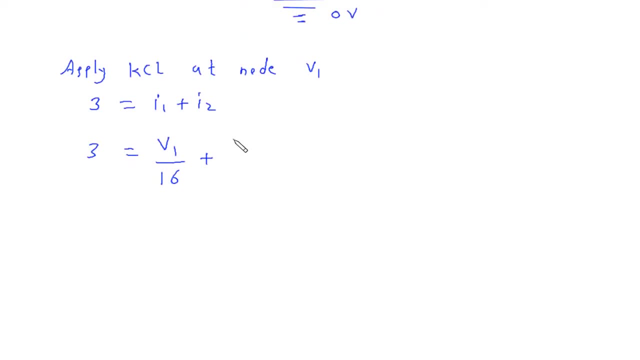 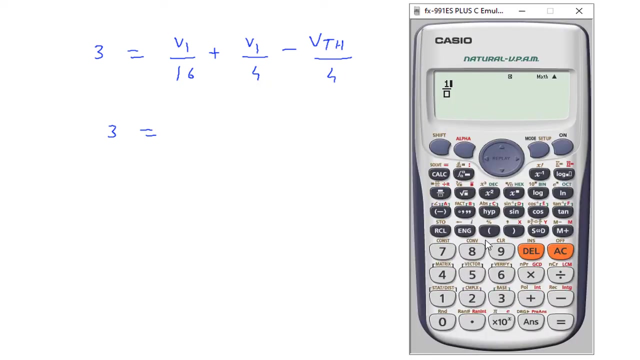 is V1 minus Vth by 4, V1 minus Vth by 4, so this will be: 3 is equal to V1 by 16 plus V1 by 4 minus Vth by 4, so 3 is equal to 1 by 16 plus 1 by 4, 1 by 16 plus 1 by 4, so 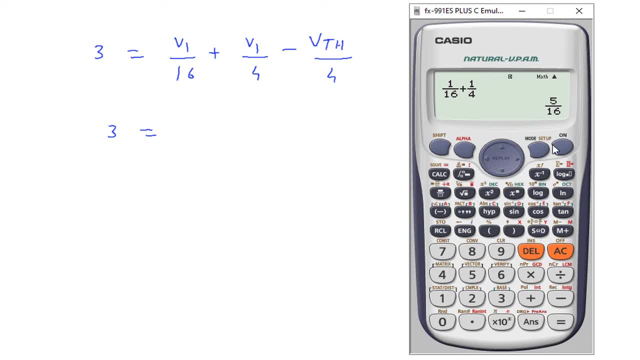 3 is equal to 2 by 16 plus 1 by 4, this will be 5 by 16, V1,, 5 by 16 V1, minus Vth by 4, let's say this is equation number 1.. 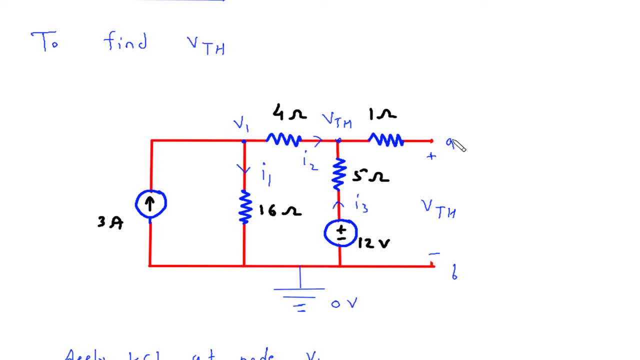 Now we will apply KCL at node Vth. Apply KCL at node Vth: 5 by 16, V1, 5 by 16 V1 minus Vth by 4, let's say this is equation number 1.. Now we will apply KCL at node Vth. 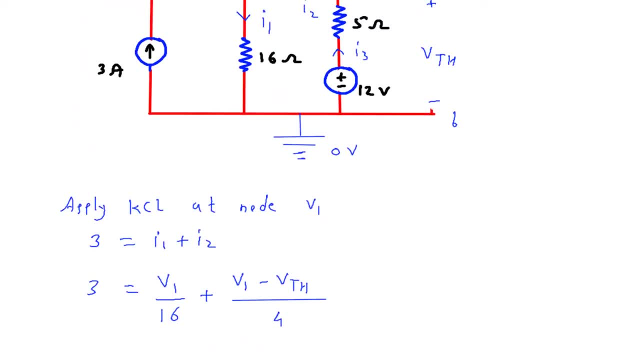 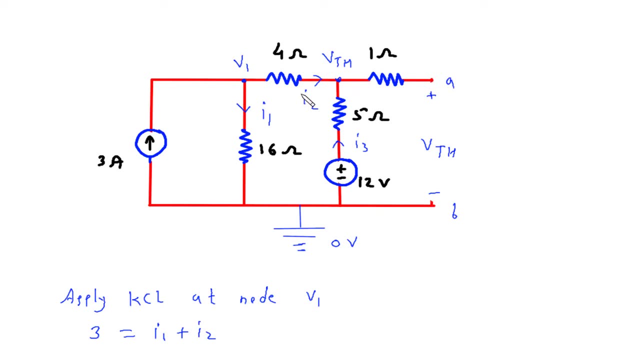 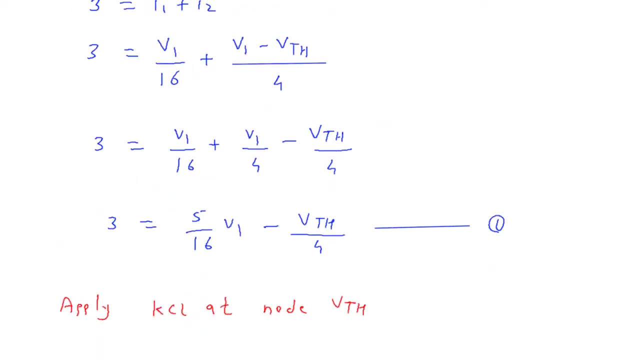 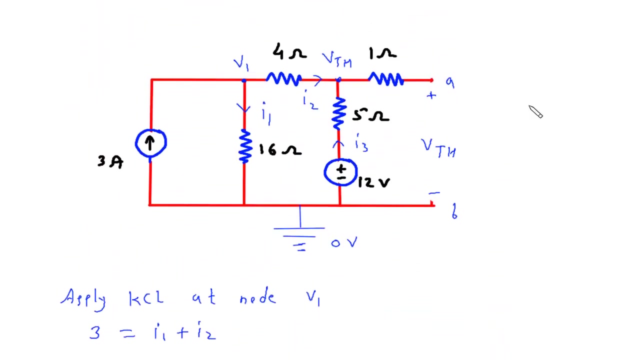 So entering current at this node is I2 and leaving current is I2 and I3 is the entering current I2 plus I3, I2 plus I3 is equal to 0, I2 plus I3 is equal to 0, now I2 is I2, is V1 minus. 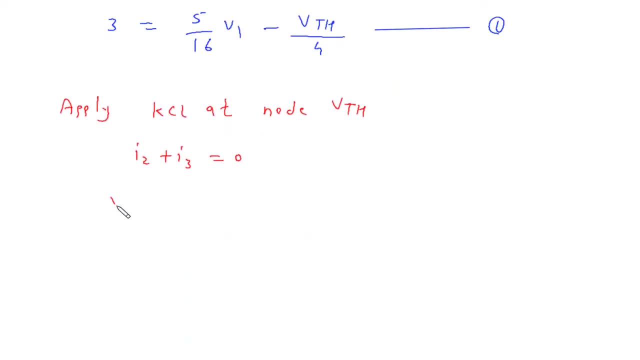 Vth by 4, V1 minus Vth by 4 plus I3, I3 is 12 minus Vth, 12 minus Vth by 5.. Ich equal to 0. So this will be V1 by 4 minus Vth by 4 plus 12 by 5 minus Vth by minus Vth by 5 is equal. 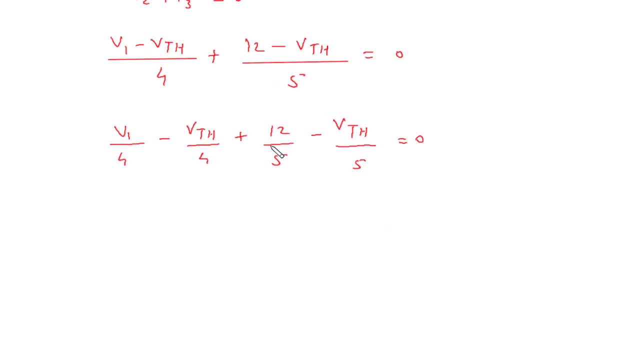 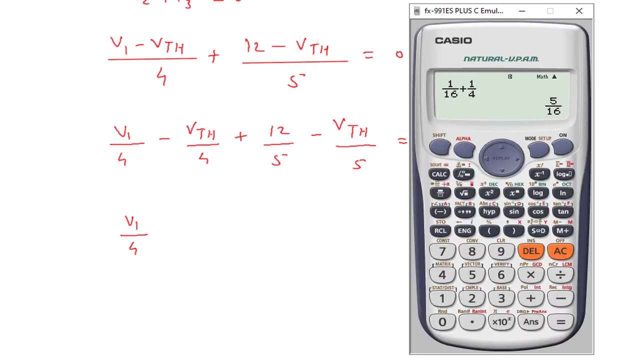 to 0. So this will be V3 minus Vth by 4, plus V2 minus Vth by 4, plus Vth by 5, minus Vth by V1 by 4, and this will be 1 minus 1 by 4, minus 1 by 5, minus 1 by 4, minus 1 by 5. 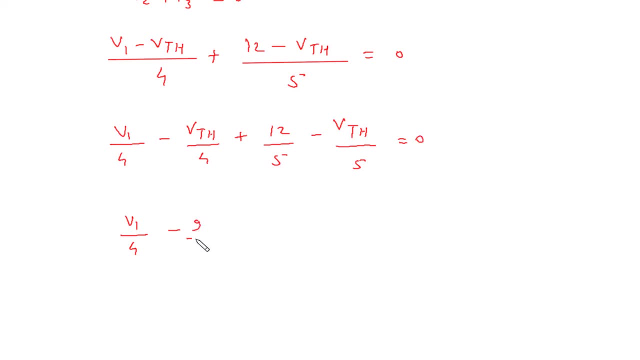 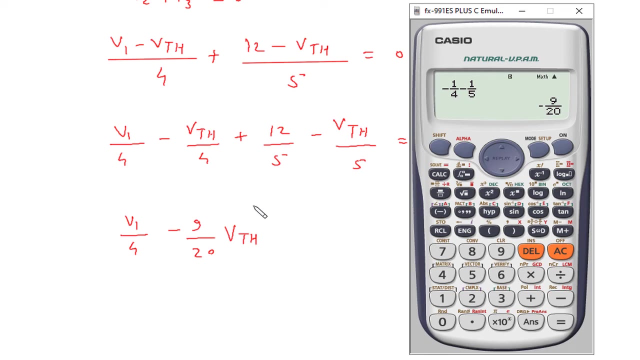 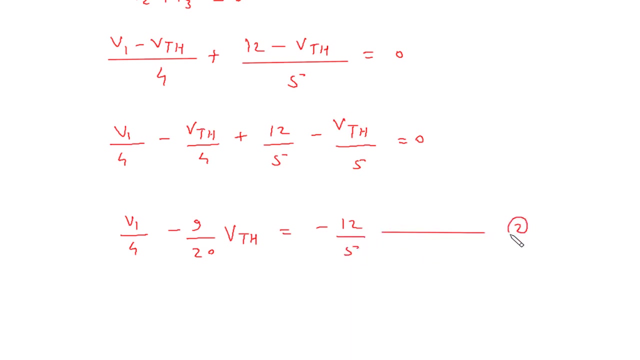 so minus 9 by 20, minus 9 by 20, Vth then is equal to this will be minus 12 by 5. let's say this is equation number 2. now we have equation number 1 and equation number 2, so solving: 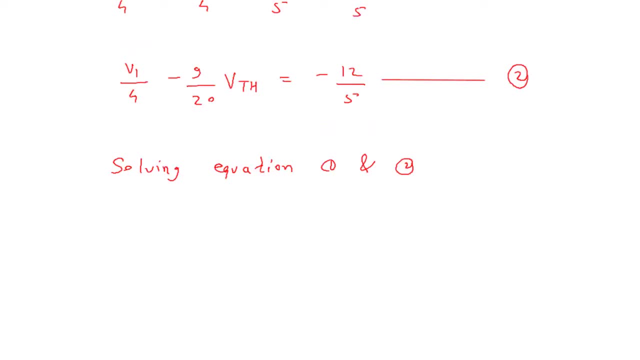 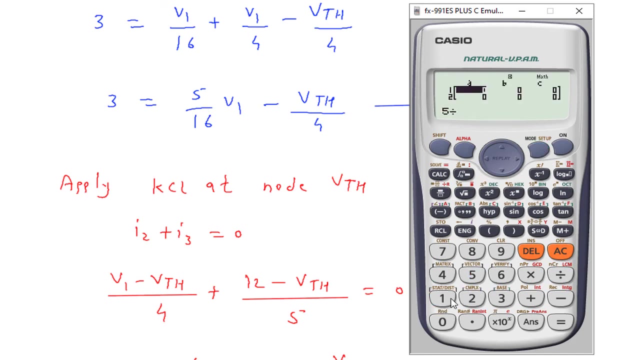 equation 1 and 2, we get mod 5, 1 and we get this will be 5 by 16. then minus 1 by 4 is equal to 3. then from equation 2, this will be 1 by 4 minus 9 by. 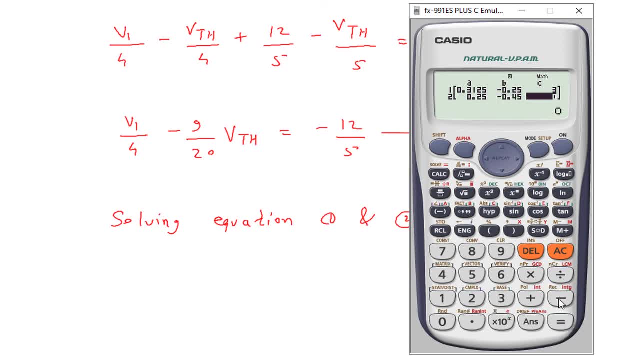 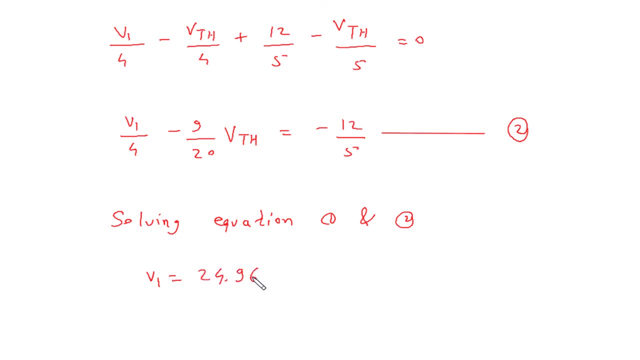 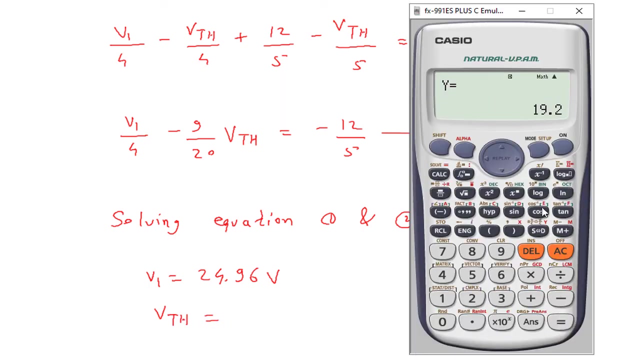 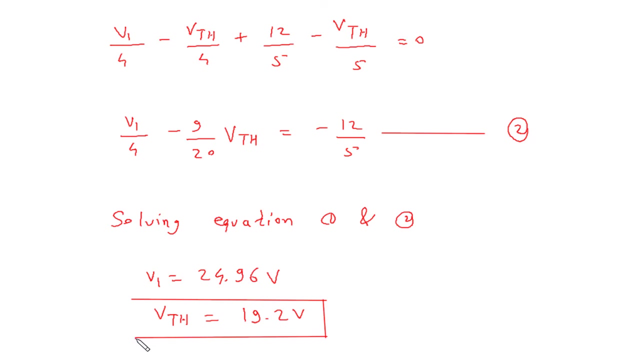 20, then minus 12 by 5. so this is: V1 is equal to 24.96, V1 is equal to 24.96 volt and Vth is equal to. Vth is equal to 19 point 19.2 volt. so this is the value of Vth and Rth is 5 ohm from this. 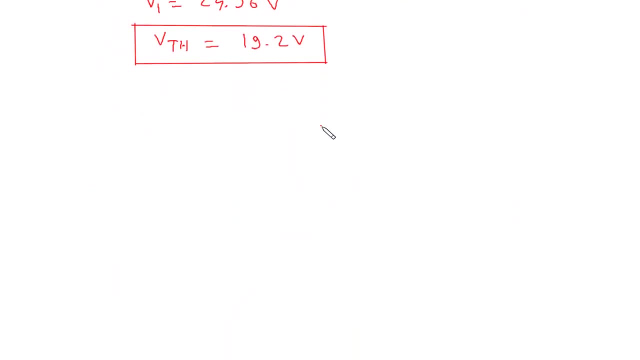 we can draw Thevenin equivalent circuit. So this is the value of Vth, and Rth is 5 ohm. from this we can draw Thevenin equivalent circuit, so Thevenin equivalent circuit will be resistor and voltage source in series, so this will be Vth. 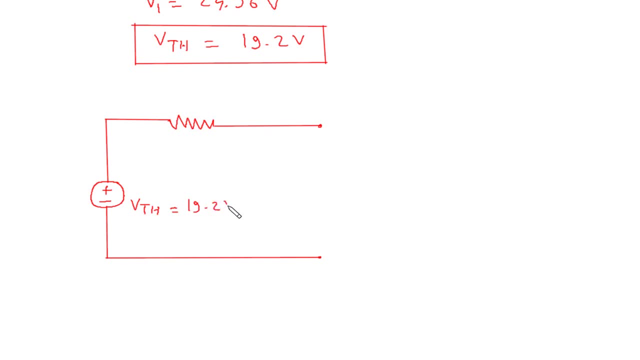 Vth is equal to 19.2 volt and Rth is equal to 5 ohm. Rth is 5 ohm. What we have to find, We have to find. Vth is equal to 19.2 volt and Rth is equal to 5 ohm. What we have to find, We have to find. 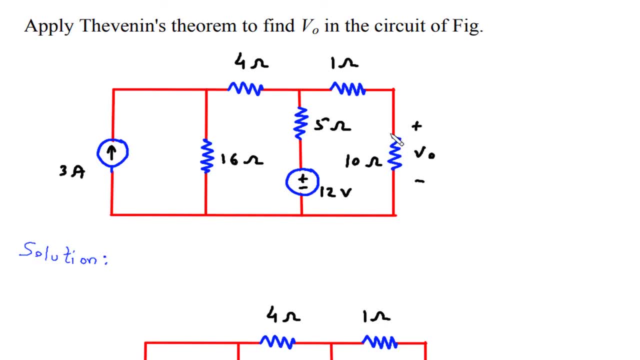 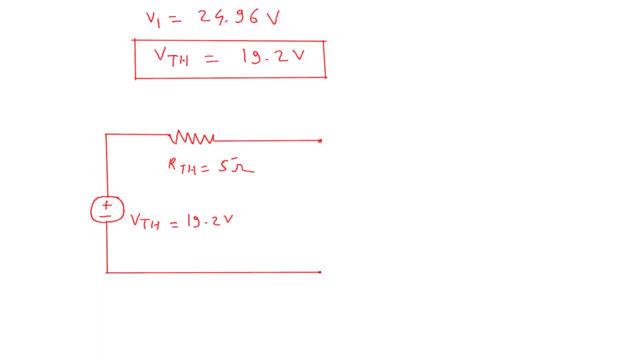 Vo this Vo voltage across this 10 Ohm. now we will put this 10 Ohm back, so here this will be 10 Ohm resistor, this will be plus, minus Vo and this is 10 Ohm. now, here we can. 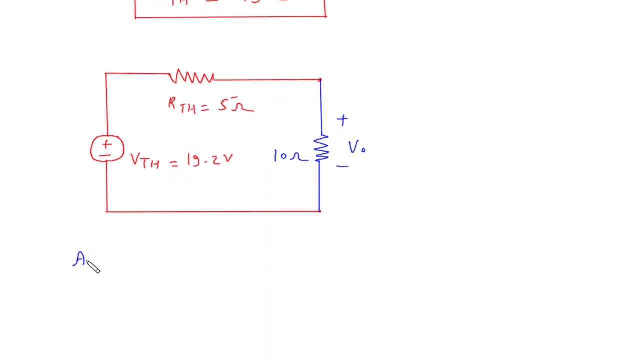 apply voltage division rule. so by applying voltage division rule, Vo is equal to. Vo is equal to this voltage, 19.2 into this resistance, which is 10 Ohm divided by 10 plus 5, so this will be 19.2..